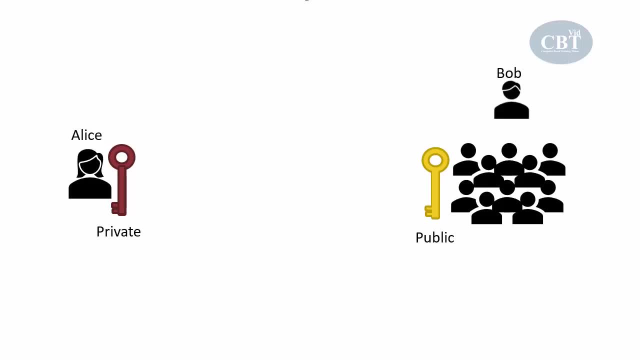 to exchange some data with Bob. So she provides Bob with her public key and asks Bob to encrypt the message using her public key and send it back to her. So Bob has a clear text, a plain text, And he uses Alice's public key, encrypts the message and then forwards it to Alice. 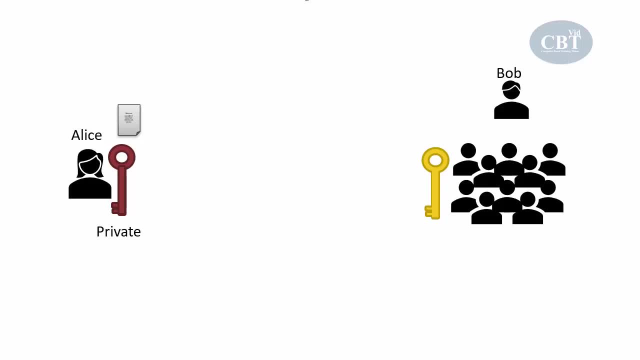 Now this message that has been encrypted with Alice's public key can only be decrypted with Alice's private key. Remember I said, if you encrypt the message with one key, you can decrypt it with the other key only and not any other keys. So even if the whole crowd has Alice's public key, 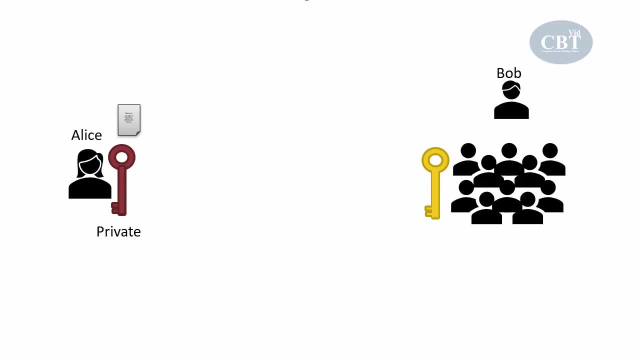 cannot decrypt the message that was encrypted with Alice's public key, So Alice is the only one who has the private key. She can decrypt her message using her private key and see the content of the message. Now, what if Alice encrypt the message using her private key? 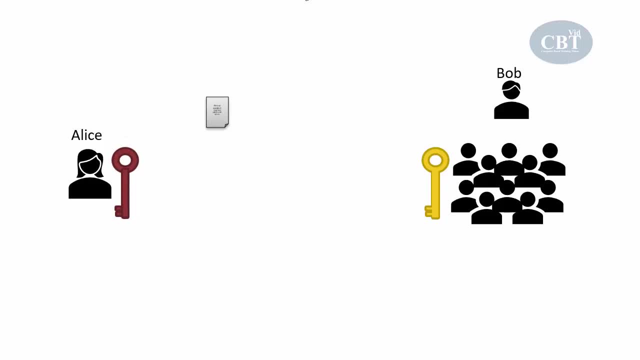 So when she encrypts the message using her private key and forwards it to Bob, who can decrypt that message? Well, Bob can use Alice's public key and decrypt the message. so can the rest of the public. So what's the point of encrypting that message? 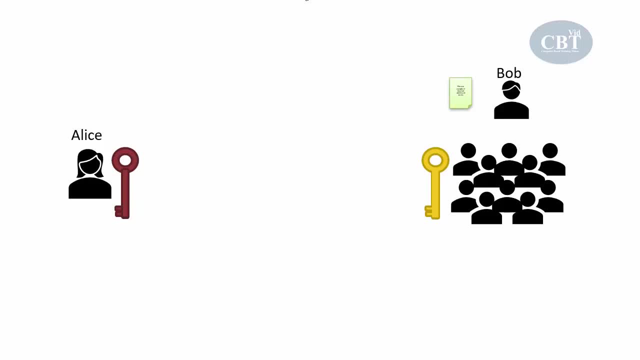 if everyone can decrypt that message and see the content of the message. If someone encrypt the message using their private key, the whole concern is not the confidentiality of the message. So the concern is not really encrypting the message so that no one can see the message. 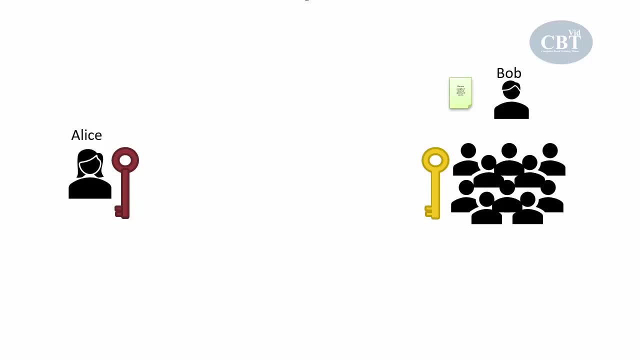 The concern is to make sure that the message came from that person, from the right person. So in this case, if Bob asked Alice to encrypt the message using Alice's private key, that means Bob doesn't really care that anybody sees the content of the message. 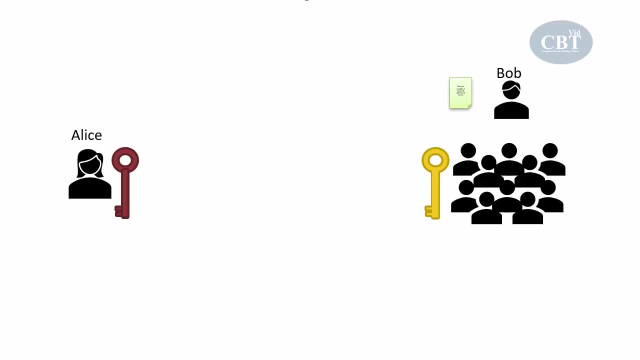 What he cares here is that the message came from Alice and no one else. The whole concept is something like when you sign a check and you give it someone to take it to the bank and cash it, the bank doesn't really care how many people have seen that check.